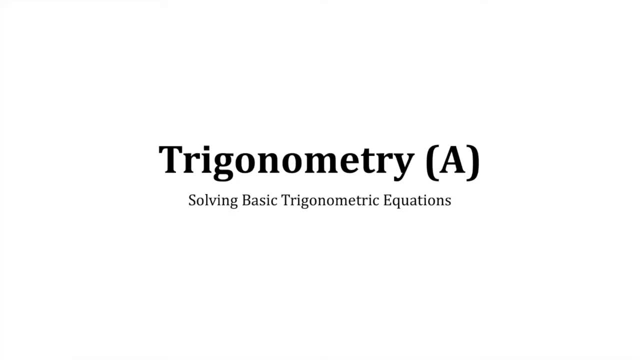 In this lesson we're going to learn how to solve basic trigonometric equations. Now most of this should be revision from last year, from National 5. 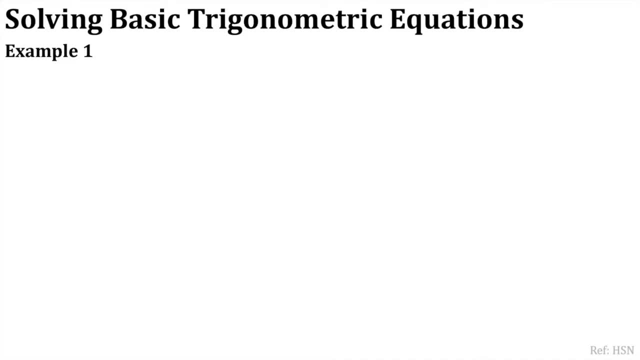 So let's just take a look at some examples because we've already covered all of the prerequisite knowledge in the previous lessons for this. So you'll be using either the graphs 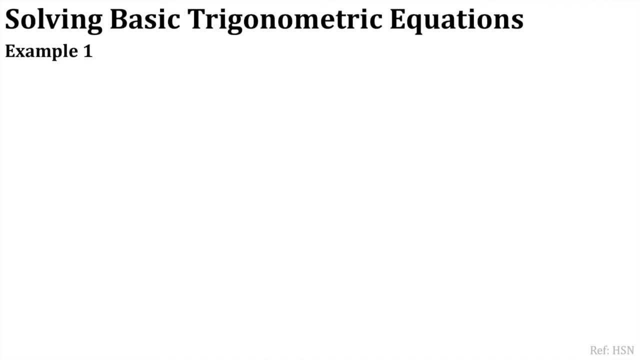 or the cast diagram to answer these questions as well. So example one, solve sine x, and you can see we're working in degrees, equals a half for x line between 0 and 360. So we could firstly 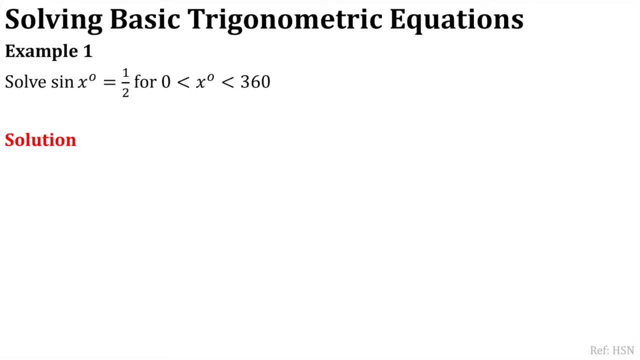 look at the graph. So if you know what the sine graph looks like, write down a quick sketch, and 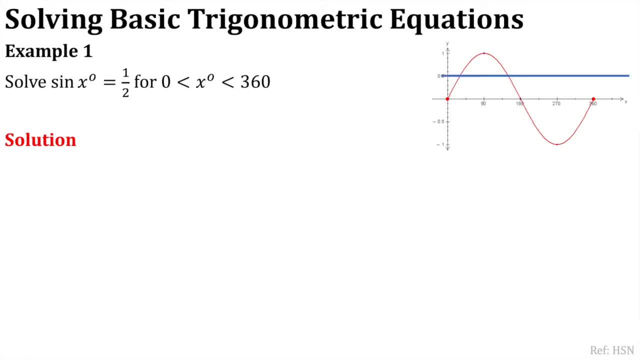 well where is sine x equal to a half? So we can put in the line y equals a half, and we can see there that that line cuts the sine curve at two points, and that's between 0 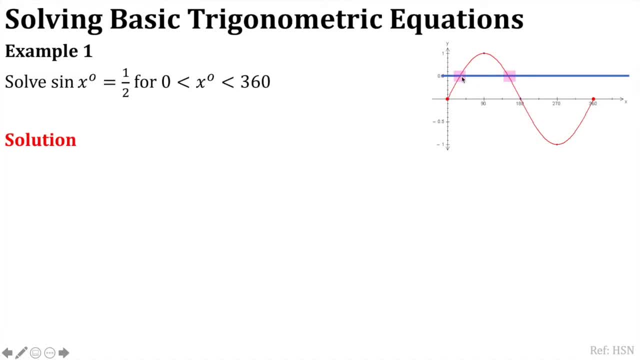 and 360. So we're expecting two answers here, one here, and one here. So this is x equals something, and x equals something here as well. Now you might immediately realise, well we've 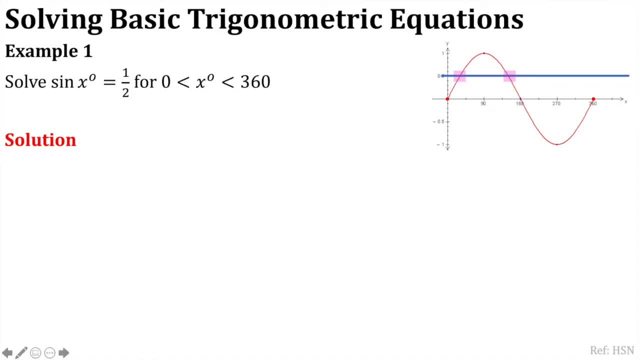 written out a sine of 30 as a half, that was one of our exact values, so that will hopefully help you here as well. So we'll have a look at some working. So if you're happy using the graph, 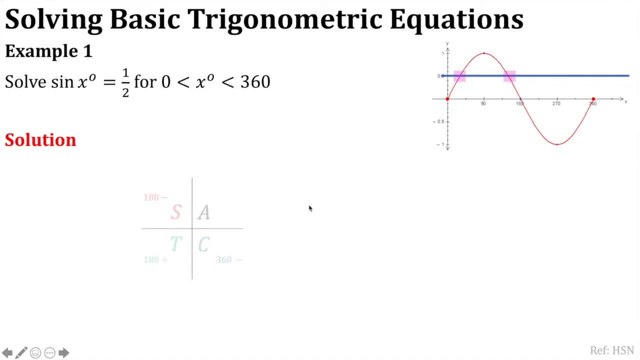 that's fine, but if you want to use the cast diagram as well, that's also fine. 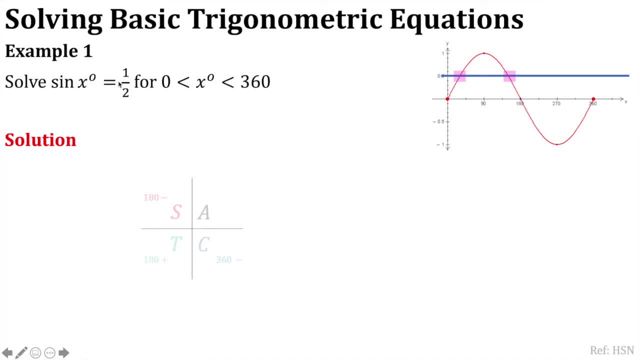 So we know that sine x is positive here, and sine x is positive in the first and second quadrants. So the inverse of sine of a half is equal to 30, like I've already said. So in the first quadrant, the answer is 30 degrees, and in the second quadrant, it's 180 minus 30 degrees, which is 150. So our solutions here then are 30 and 150. So we should be able to calculate this one. So we're going to take our solution here, 150. And we can see from the graph that that's quite possible. We can see that our answers had to lie between 0 and 45. So that one in there, and that's a 30. And between 100 and 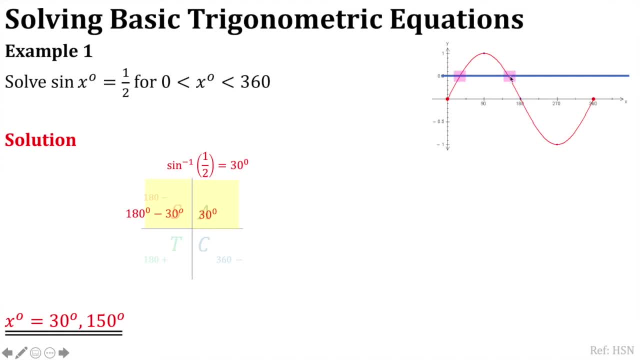 35 and 180. So again, we can see that that's 150 in there. So just now would be a good time to pause the video and copy down example one. Okay, welcome back, folks. Let's look at 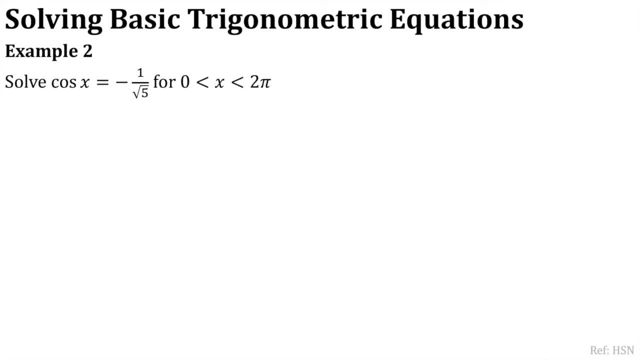 example two then. So we want to solve cos x equals negative one over root five for x lying between zero and two pi. So you can see this time that we are working in radians. So like I've said before, it's very important when we're working in radians to stick to working in radians, don't. 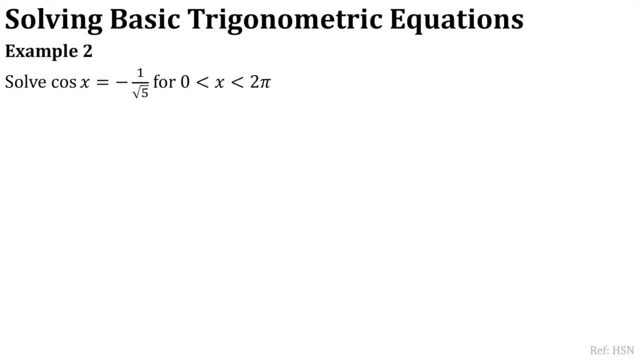 Don't ever convert it to degrees and then back again. Because if you forget to cross that out in the exam, you do lose marks. So the solution then, if we firstly just really look at the graph. 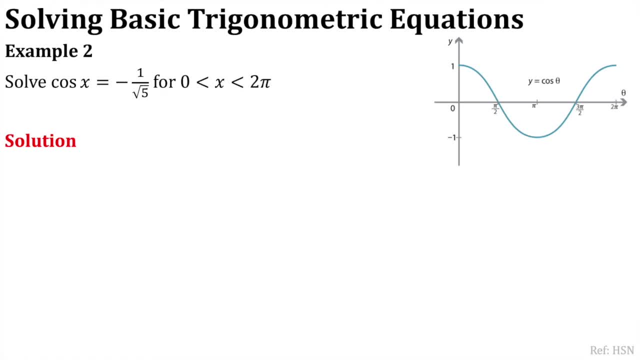 So here's the cos graph, which is lying between zero and two pi. And if I just draw in the line y equals negative one over root five, that's around here. 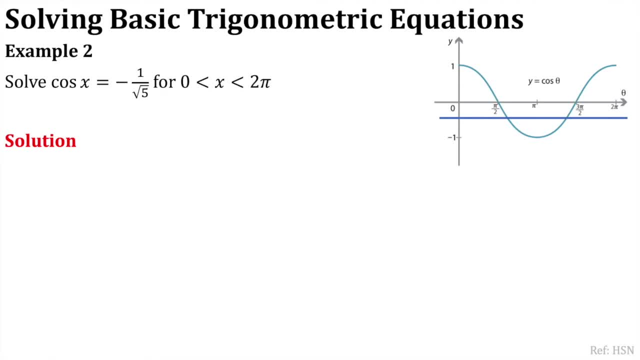 Now, we can see that that cuts the cosine graph and two points, which you can see here. So let's have a look at how to go about this. We can see that the two answers are occurring in the second quadrant 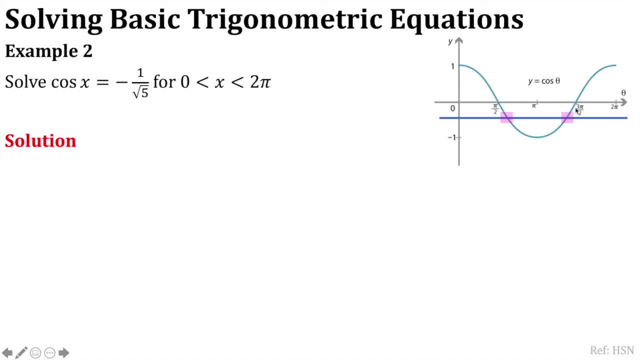 between pi over two and pi and the third quadrant. So between pi and pi over two, and that helps us with our cast diagram. 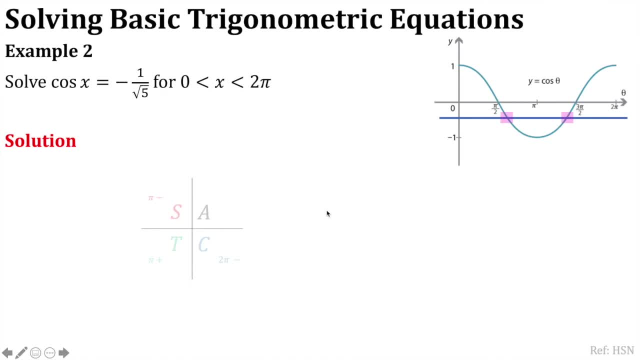 as well, remember that's where the cast diagram comes from, are the trigonometric curves to start with, so that's useful. So it's cos and it's negative, so that means that the answers are occurring in the second and third quadrants, like I said, and you can see that here. So inverse cos of positive 1 over root 5 is 1.107. Now at this point you need to 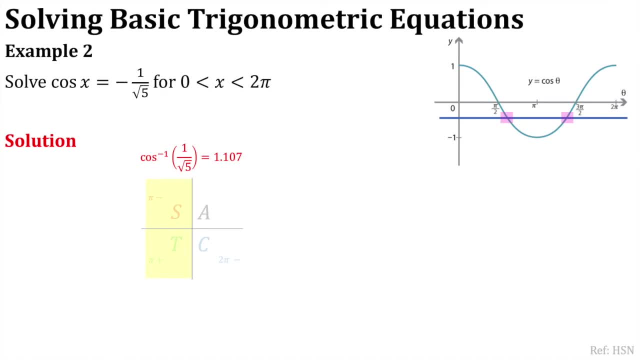 remember and have your calculator in radians, so you need to be able to change the mode in your calculator so that it's not displaying the wee d for degrees on your screen like you've always had to have up until this point when you've been working with trigonometry throughout. 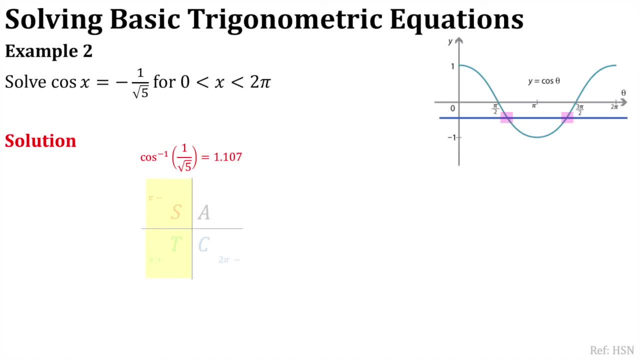 So if you're not very sure how to change that, either if you're in school, ask one of us, or if you are at home, you can maybe Google it if you don't have your calculator instructions on you. Okay so inverse cos of positive 1 over root 5 is 1.107. Now for the 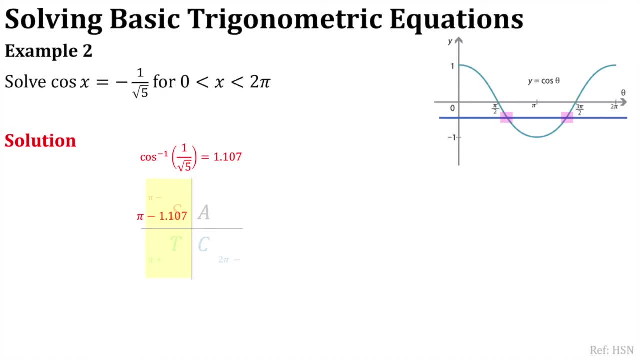 answer in the second quadrant, we need to have pi minus 1.107, and that is literally the same as the first quadrant and we're just going to have pi minus 1.107, and that's you're using the pi button in your calculator. And for the third quadrant it's pi plus 1.107. 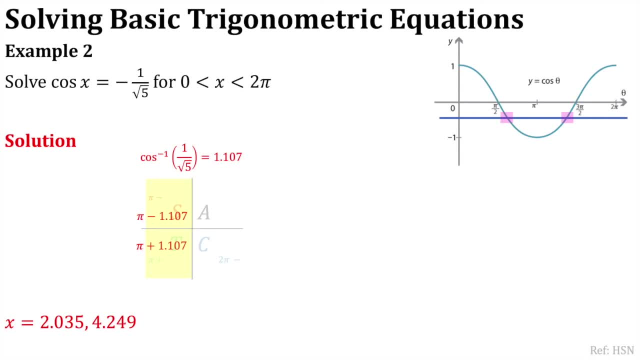 So putting those into our calculator gets us to three decimal places, x equals 2.035 and 4.249. And you can see here that one of our answers, obviously this is pi here in the middle, which is approximately 3.14, one of our answers is less than that, which is good, that's a 2.035 one, and one of them is greater than that, which is 4.249. So those 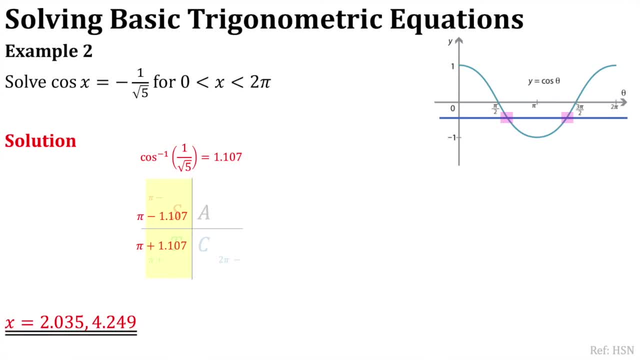 are our final answers. Now, on to example three, if you make sure you've got a wee copy of this. So solve sine x equals 3 for x lagging between 0 and 2. 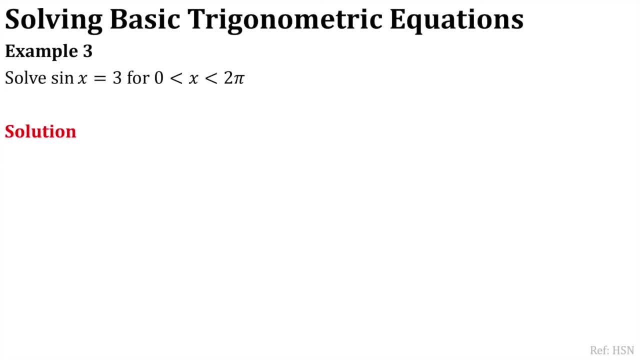 Now, if we just think for a wee moment about the graph of y equals sine x, I know this is y equals sine theta, but the same, just a different variable, same curve that we're dealing with here. Now, you can see here that that graph lies between negative 1 and 1, but we're actually looking for 2.035. 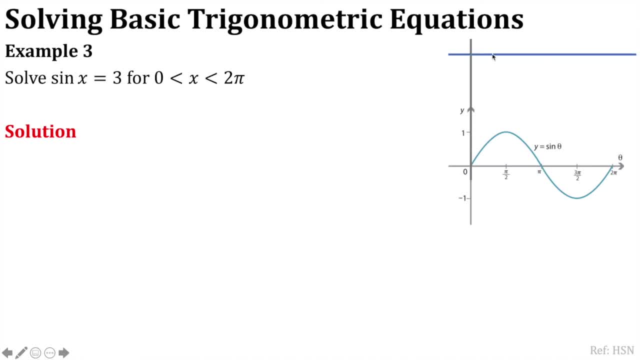 Now, if we just think for a wee moment about the graph of y equals sine x, I know this is y equals 3, so that's the line y equals 3 here, and we want to see where that line cuts the sine curve, and you can see here that that actually doesn't happen, because the range of y equals sine x, or sine theta, like I've said, is between negative 1 and 1. So there's no solution to this example. Because, as I've said, sine x lies between negative 1 and 1, so no solution here, and you have to state that. If you're asked a question like that, you need to state that there's no solution, and give a reason why. 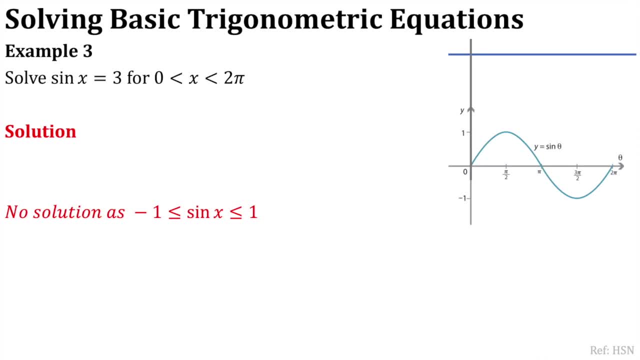 Again, folks, good ideas to copy this down as well. 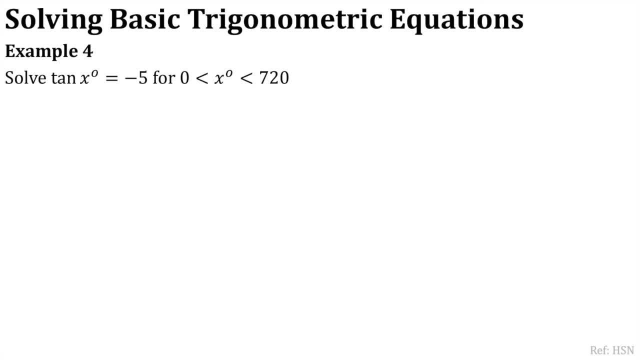 And finally, example four, so we want to solve tan x equals negative 5 for x lying between 0 and 7. 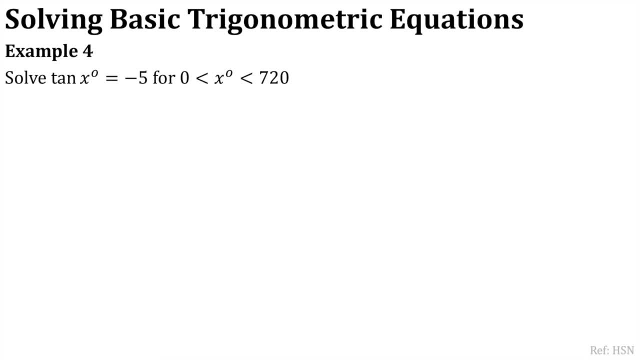 720. So I suppose, given the last example, the first thing that I might observe here is that, well the last example was sine x and we knew that there was no solution because the graph of sine x lies between negative 1 and 1. The same holds for the graph of cos 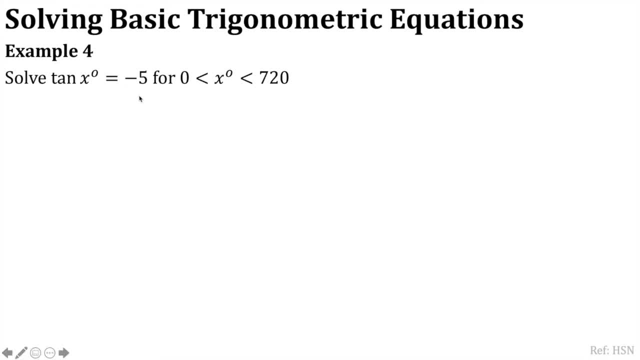 x. But tan x is slightly different, so this is okay. We can have a number less than negative 1 and greater than 1, remember, because the tan graph lies between negative infinity and infinity, so that's fine. The other thing I'm observing here is this range of values. 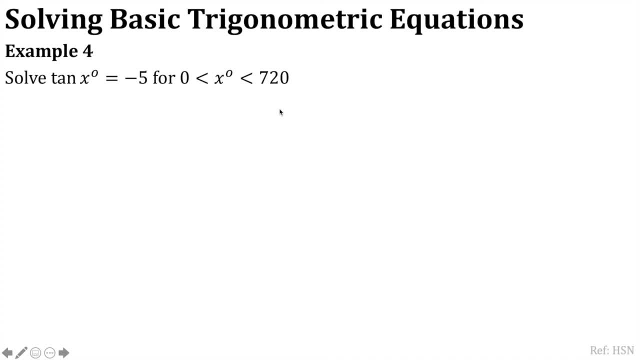 Normally I'm solving between 0 and 360, or 0 and 2pi, but this time I'm solving between 0 and 720 degrees. So that makes the question slightly different. 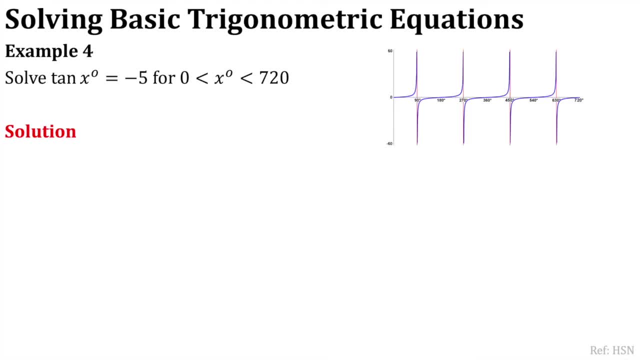 So the solution then, we'll have a wee look at the graph first, and you can see here that this graph of tan x is lying between 0 and 720. And I'm just going to put the line y equals negative 5 in. And you can see here that that cuts the tangent graph four times. So we are looking for four different answers here. 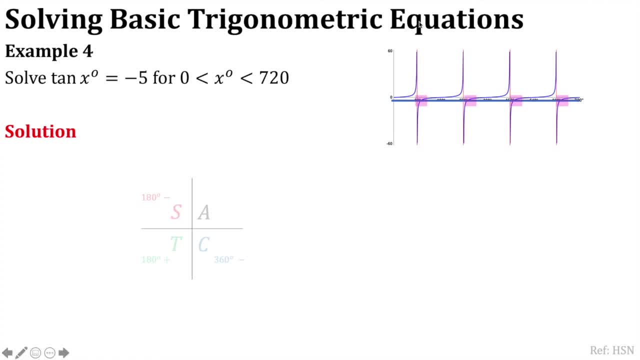 So, bring my cast diagram in. I can see instantly from the graph that one of my answers lies in the second quadrant and one of them lies in the fourth quadrant. Okay, that's for between 0 and 360. So that's the second quadrant and the fourth quadrant because tan x is negative here. It's equal to a negative number. 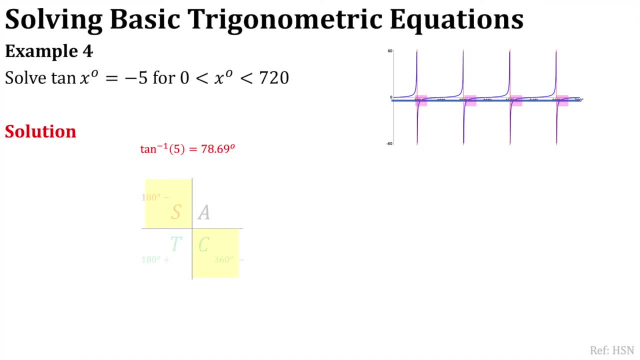 So, the inverse tan of positive x is equal to negative y. 5 is 78.69 degrees. For our answer for the second quadrant, that's 180 minus 78.69. And 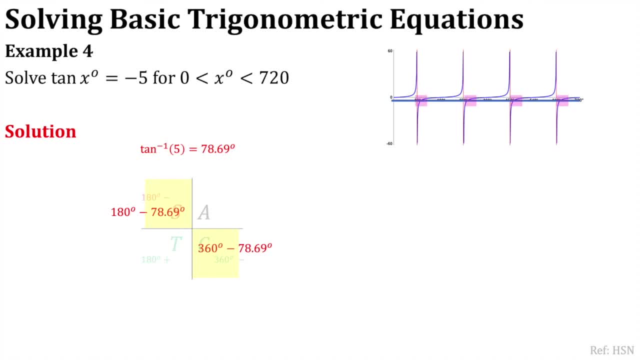 for the fourth quadrant, 360 minus 78.69. So those two answers are 101.31. And we can see that is just past 90 and no more. So that's around the correct place. And 281.31. And again, that's just past the 270 mark there. And that red line is 270, remember, the asymptote. 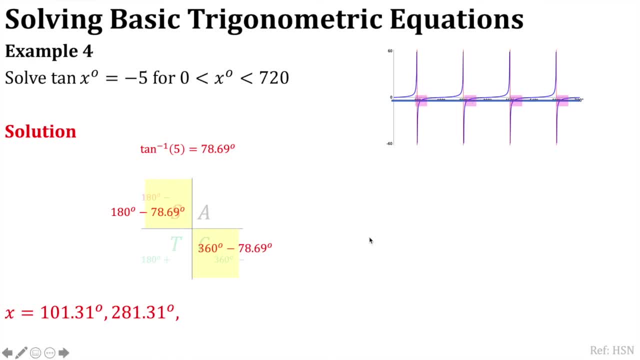 So now we do have two other answers to get as well. So if we just look at this one here, 101.31. 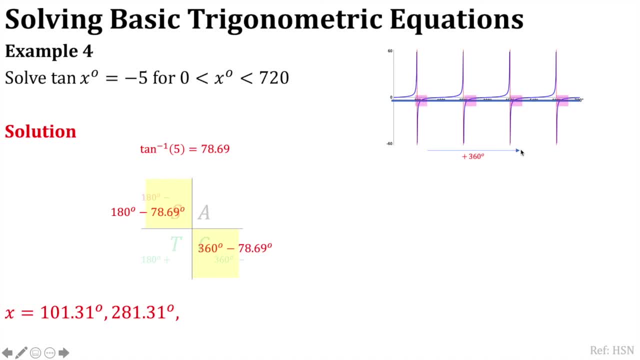 If we add 360 on to that, that will get us this answer here. And that's 461.31. Because remember, the graph repeats itself. So all of the graphs of the trigonometric functions all repeat themselves after 360 degrees, if it's just a single angle here. Okay, for the second answer, 280.